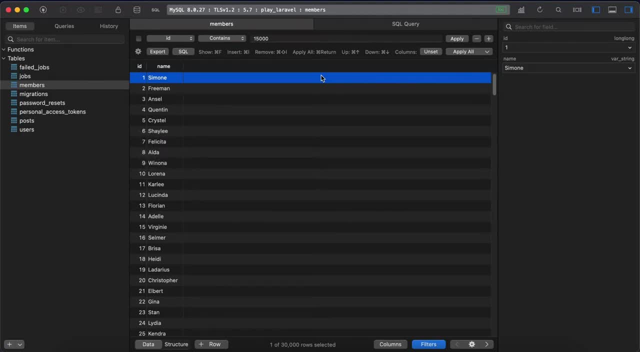 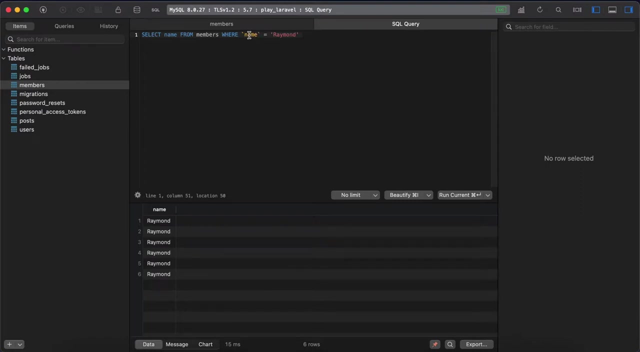 in this lesson we will learn how database index affects on our application performance. let's start here. in our members table I created 30,000 row with ID and name. if we do query here for filtering users by name or members by name here, excuse query, it takes 16 millisecond. run it again. 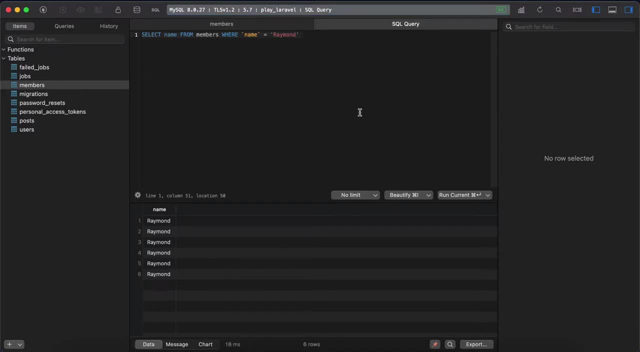 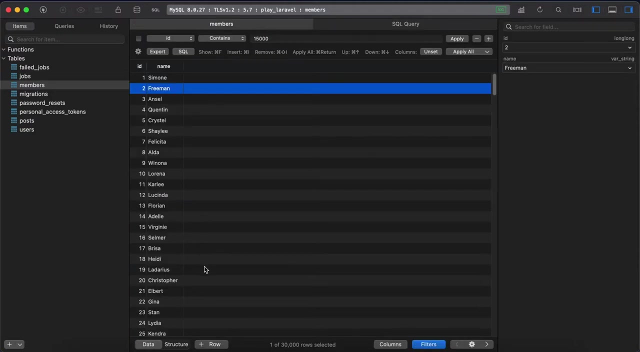 18 millisecond. it's fast, but not enough. again it's 17, but when we try to find it by ID right, where ID equal to 20,000, for example, it takes half millisecond or 600 microseconds right. the reason behind that: if we go to our table structure here we have an index created on 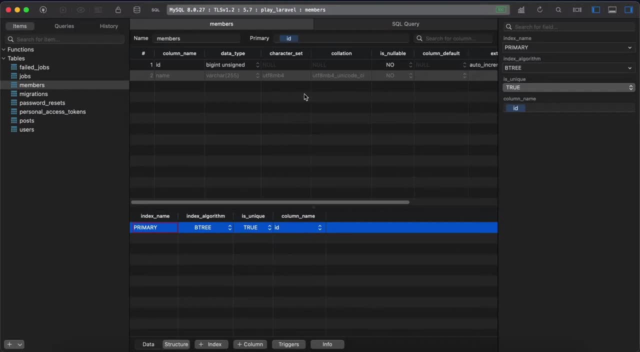 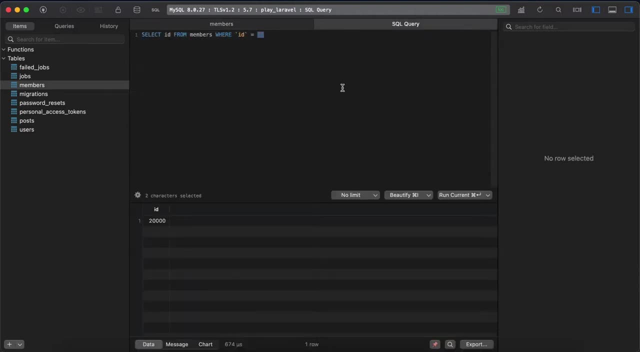 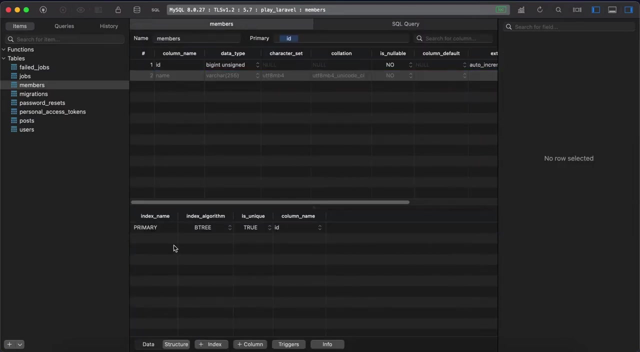 ID column right. so to make it works with name column, we need to create an index for our name column. let's try again with our name column here and to check results. yeah, now execute. it works and it takes again 80 milliseconds. so now let's create our index on name column here in our table. 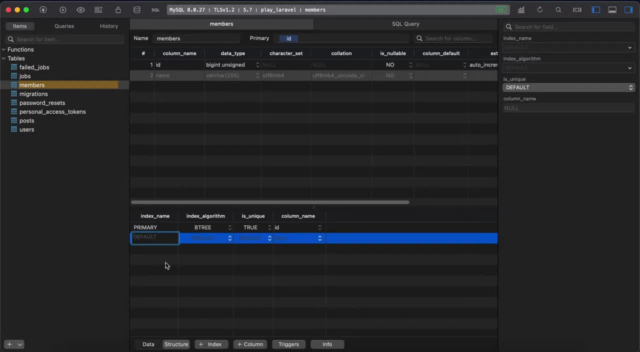 structure. our index name will be, for example, members name and our algorithm will be B three and name values is not unique, so it's false and our column name is our name, this one here. right name control S in my table plus and this back again. so here it. 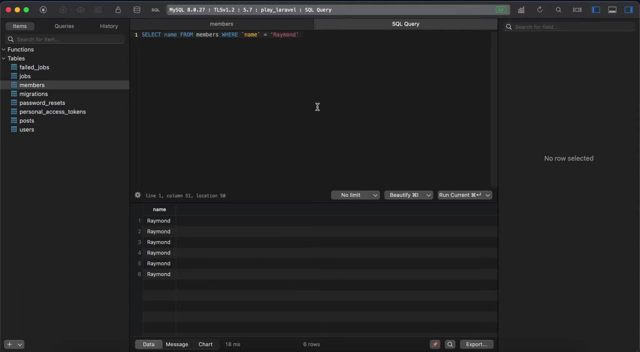 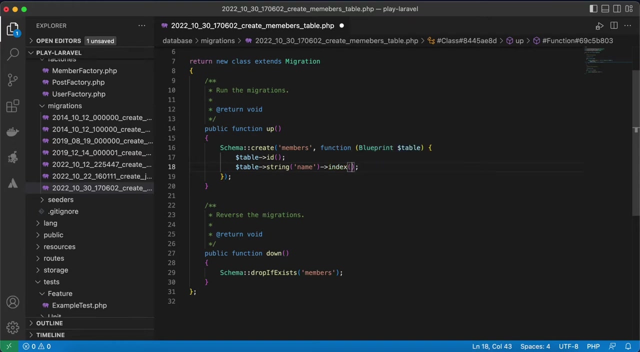 takes 80 milliseconds. now when we try it after indexing, it takes 800 microseconds super fast to create index using laravel migrations. you can use this method, index and you can pass the index name, like this one here in our cases, this one member's name, for example.